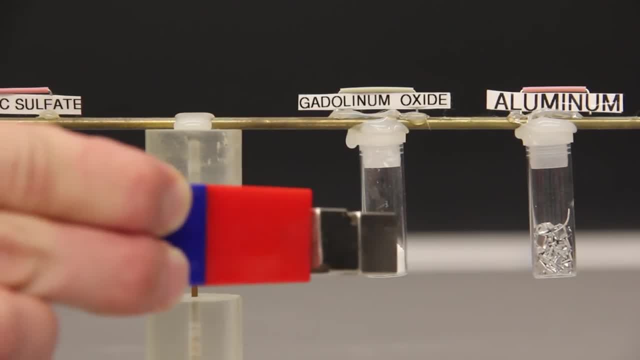 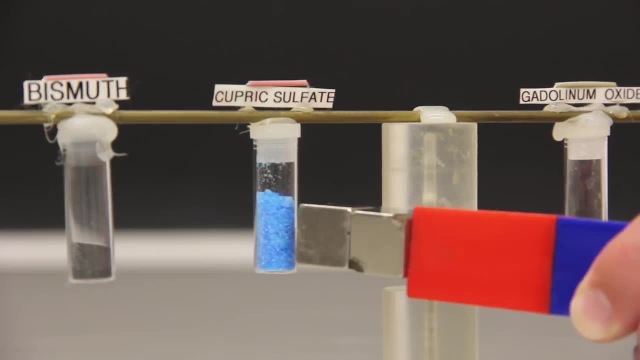 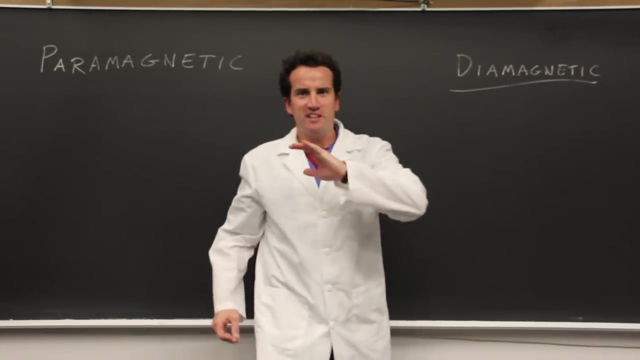 I'll explain why later. Gadolinium oxide and cupric sulfate are good examples of paramagnetic substances. Cupric sulfate is a salt that can be picked up by a magnet. Diamagnetic materials are exactly the opposite of paramagnetic: They are always repulsed. 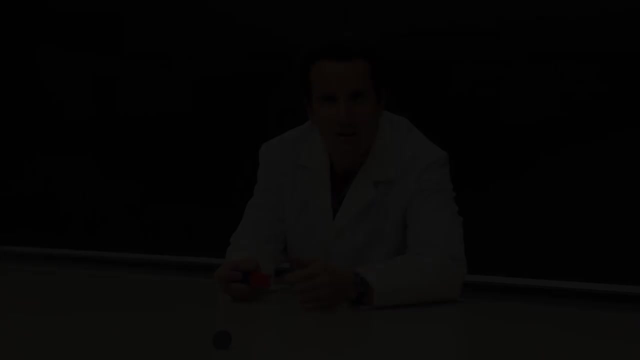 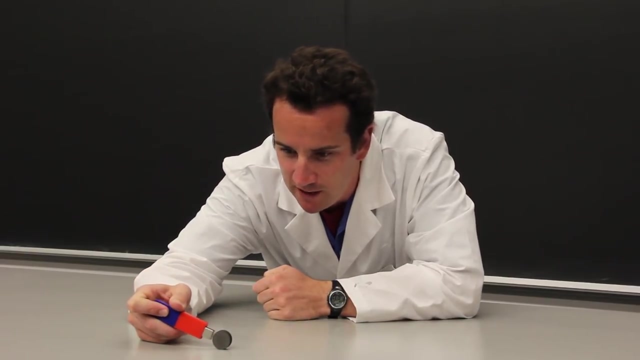 They would rather die than be in a magnetic field. An important example of a diamagnetic material is graphite. This specially made pyrolytic graphite is repelled by a magnetic field. Don't be confused: This is not static electricity or eddy currents. 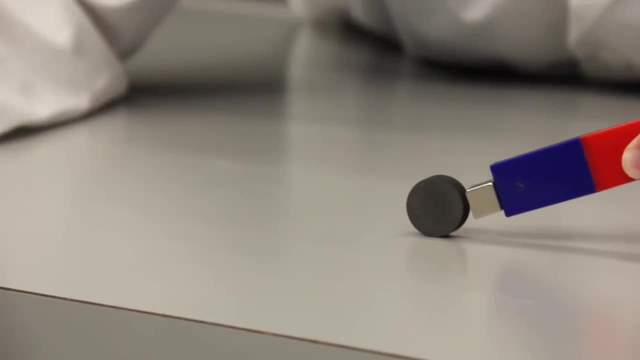 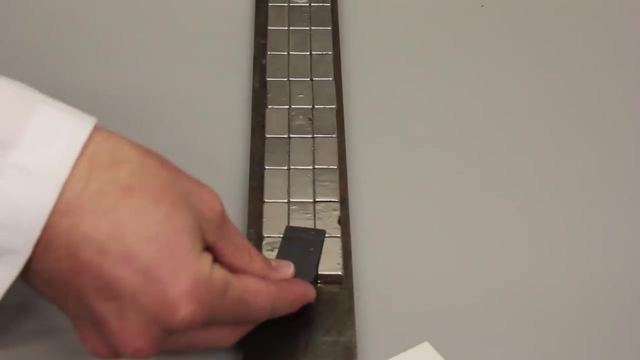 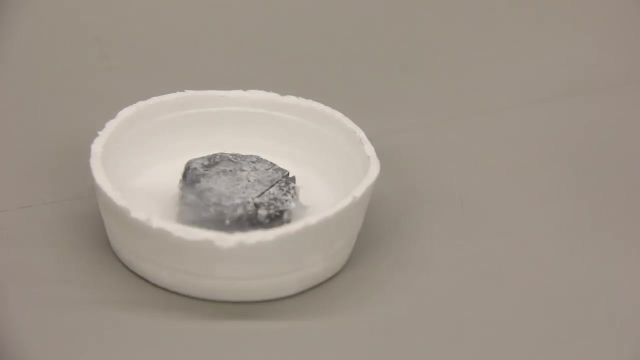 Graphite is repelled by a magnet, always both by the north and south end. Pyrolytic graphite is a grown crystal of flat carbon layers which maximizes the diamagnetic effect. Of course, the best diamagnets are superconductors. 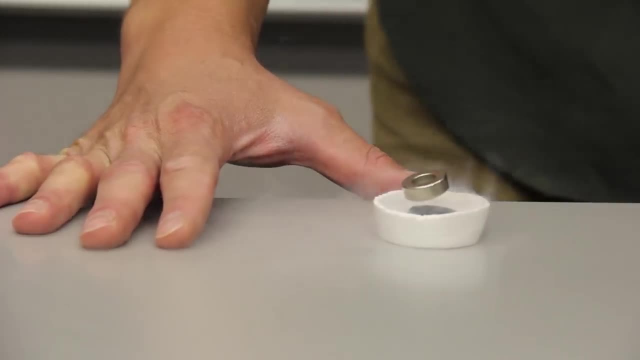 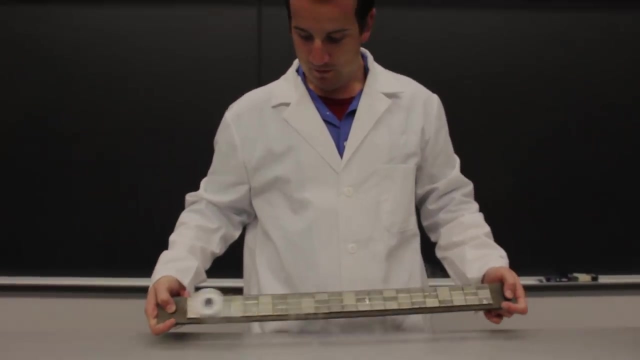 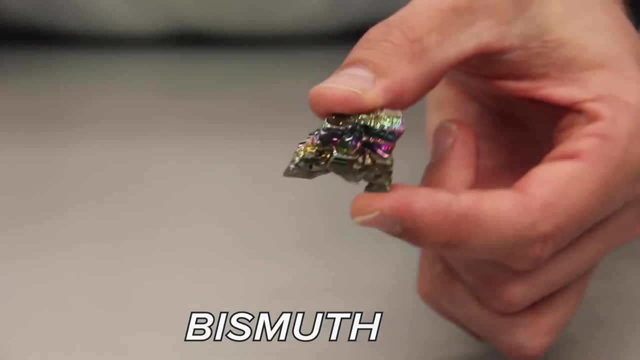 which, at low temperatures, provide exact opposite repulsion to whatever magnetic field is present. when they're chilled, They are perfect diamagnets. The most famous and powerful diamagnetic is bismuth, element number 83 on the periodic table. The bismuth-powered boat sails toward the weaker magnetic fields. 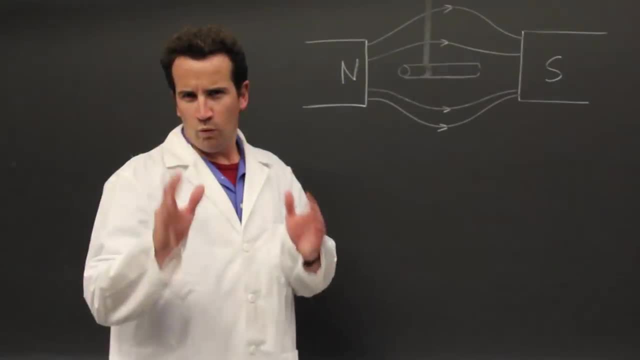 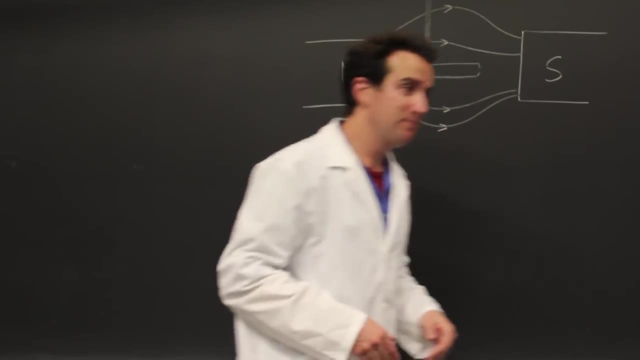 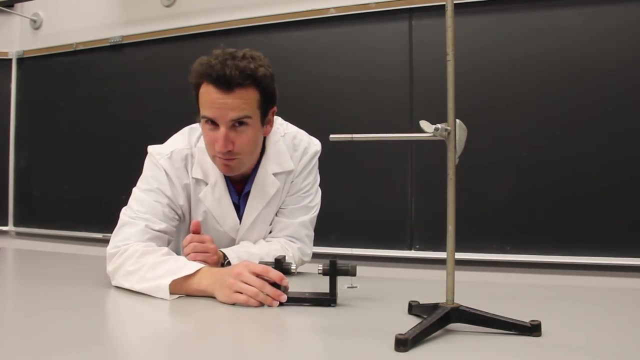 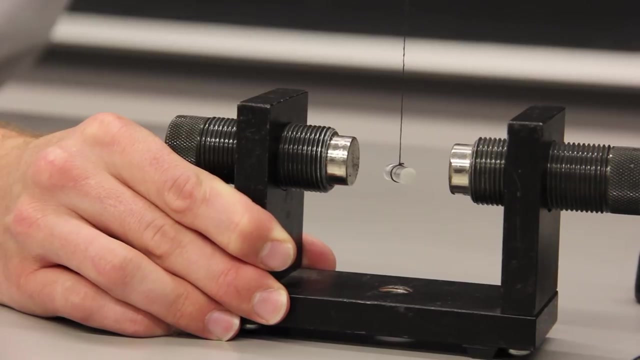 One way to check whether an object is diamagnetic or paramagnetic is to see how it aligns itself in a magnetic field. Diamagnetic objects like glass will rotate to avoid magnets. Here we see that the glass is diamagnetic because it twists to get to the weaker magnetic field. 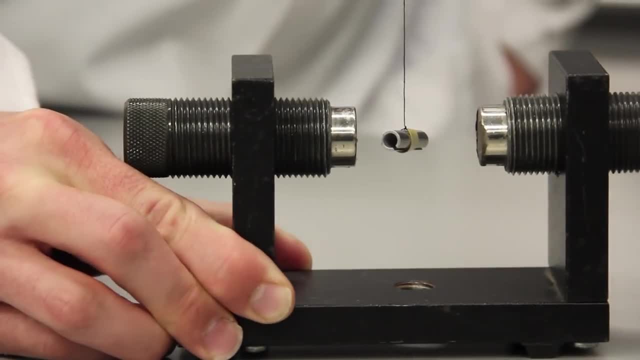 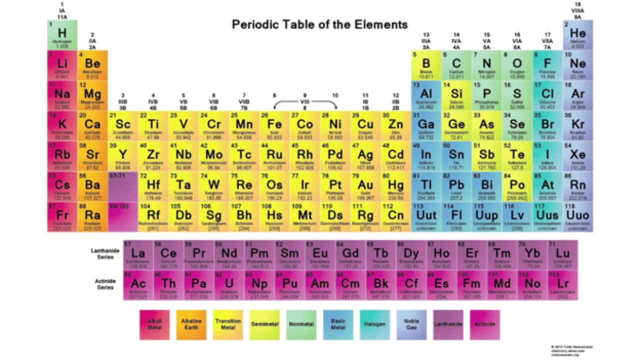 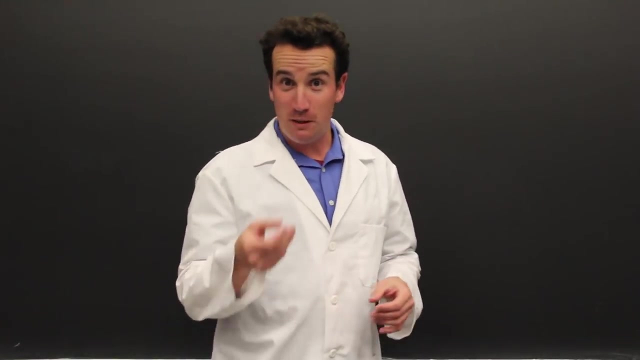 But aluminum rotates into the field typical of a parallel paramagnet. On the periodic table we see that aluminum has three valence electrons. So what does it take to understand what it means for something to be a paramagnet or a diamagnet?